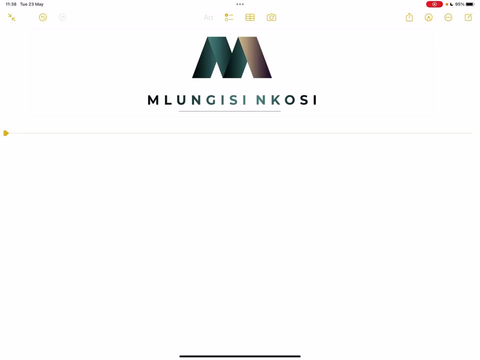 all, right, so we're going to be talking today about electrostatics, right? so, as I said, so we'll be looking at this section just a little bit more broadly as we go along, right? so this will be lesson one. of course, another lesson will come, and until we conclude this, 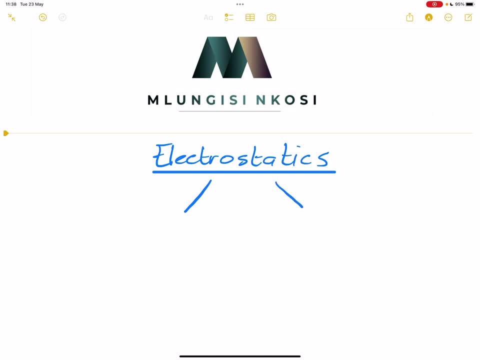 section, right? so first of all let's look at electrostatics. so electrostatics comes from a compound word meaning electricity, right? so we're looking at movement of charge in this case, and statics means that that is stationary and that means electricity that is not in motion. so there. 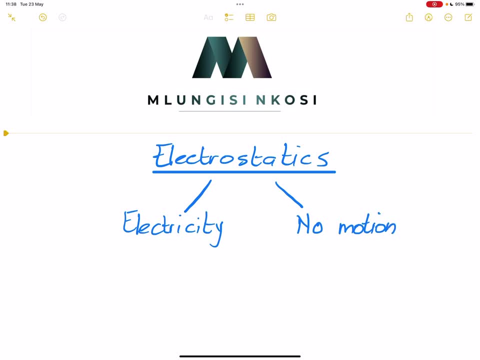 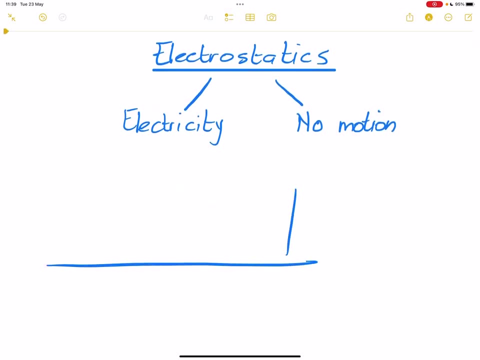 is no motion here, all right. so I mean, one day you're moving on a carpet, you know, across the carpet floor, and as soon as you touch the doorknob- right, especially in winter- right, if you're walking across that carpet, as soon as you touch that doorknob, oh tick, there's that surge of electricity. 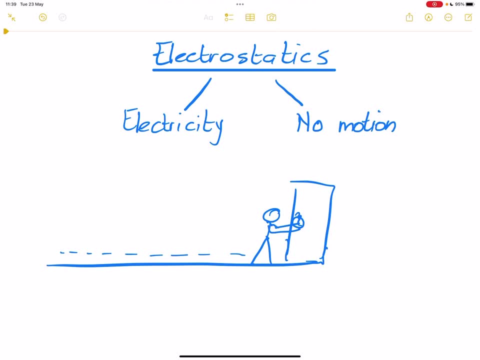 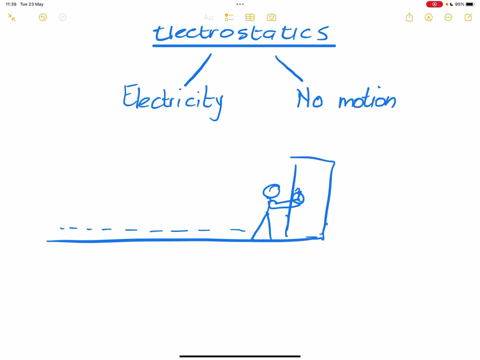 you know, just um, you know, you feel it in your hands, right, that is called electro electrostatics, right? or you know, sometimes, if, even if you take off your jersey- okay, you can try it, especially in winter as well- when you take off your jersey in the dark, you'll see that there are little sparks that are 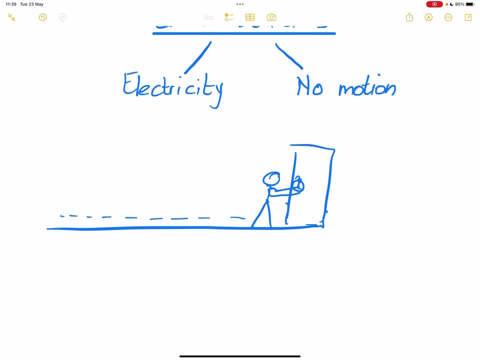 showing there and all of that is a sign that there is electricity that is not in motion, in this case referred to as electrostatics. okay, of course, some of you would have seen, when you rub a ruler, you know, on your head, okay, there's a transfer of you know charge, in that case causing obviously 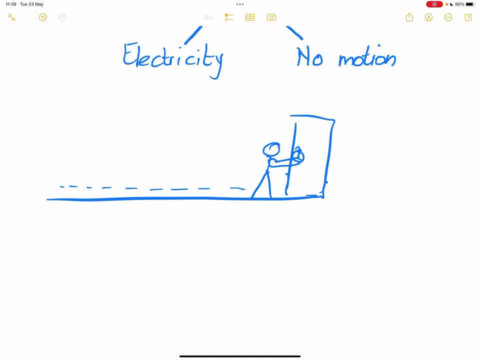 the ruler to end up with the- you know, positive charges and, as a result, it will be able to attract paper. right now, let's, let's explain what causes all of that, right? so in this case, when we talk about electrostatics, so first of all, what happens? there are positive and negative. 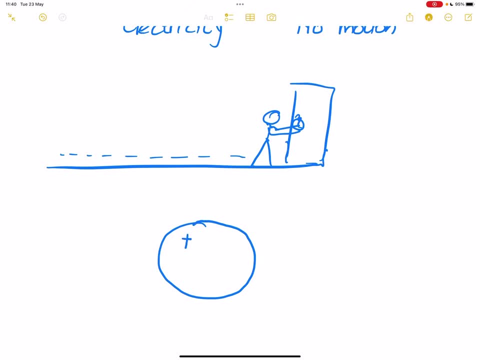 charges, charges. We usually call the positive charges protons, right, So the positive charge is called a proton right. But we also have negative charges, right, And we call the negative charges electrons right. So I'm going to put there those electrons right over there, right Now. 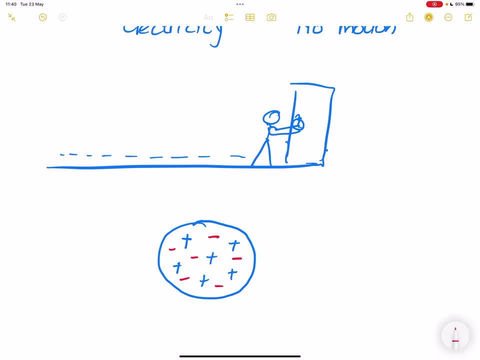 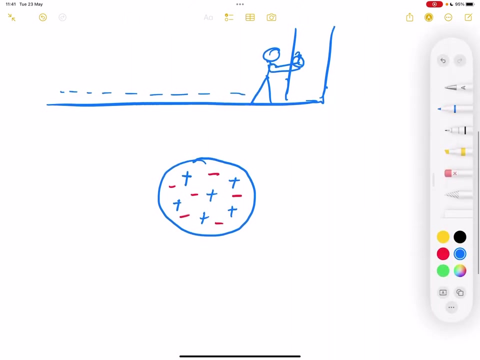 what happens when the number of protons and the number of electrons are equal, right? So, if you note there, how many protons do we have? We've got six positive charges and we also have six negative charges, right? So in this case, what happens? Well, we say this particle or this object. 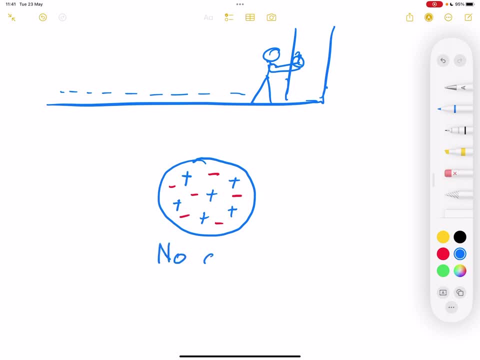 has no charge, right? So in this case we say that it has no charge. Remember what it means when we say there's no charge in this case. or we can say that it is neutral. That's the word that we use, right? So when we say an object is: 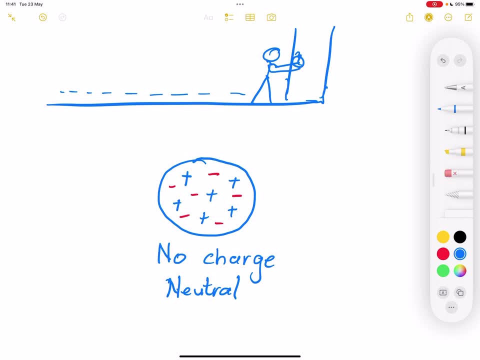 neutral. it means that the number of positive charges is equal to the number of negative charges. okay, Right Now, what happens in this case, when I can remove either a positive or negative charge? Well, I can remove either a positive or negative charge, right, So I can. 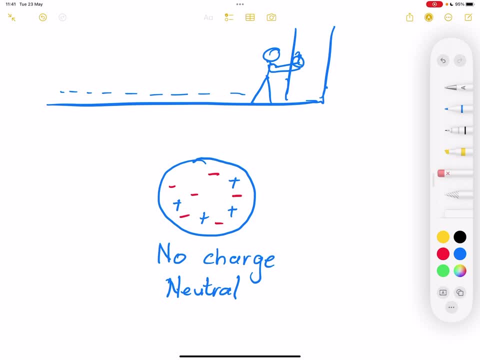 remove either a positive or negative charge. Let's remove two of those charges, right? So what happens Now? we've got an excess of electrons, right, So we've got more negative charges than we do positive charges, right? Or we can say: well, we've got a deficit, a deficiency of positive. 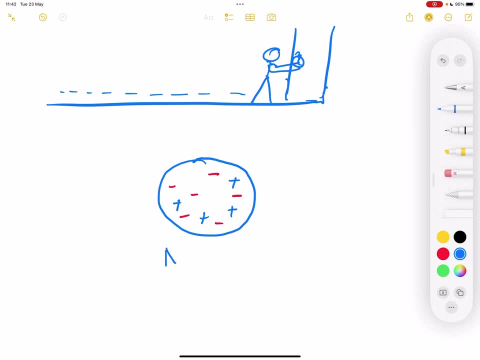 charges. So, as a result, this guy becomes negatively charged. I want you to please remember that. So when I say that an object is negatively charged, I do not mean that there are no protons, but what it simply means is that there are more electrons than there are protons. okay, Right, I. 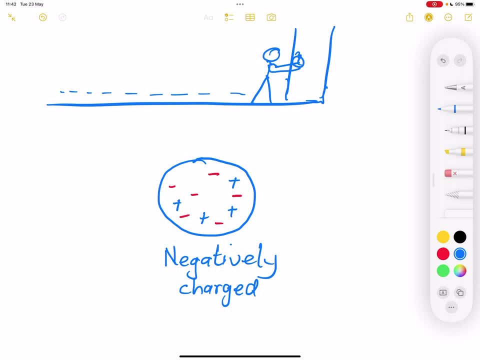 hope that makes sense, ladies and gents, But similarly, let's just try and get these back again. So, if I can put in now, let's get some more protons into this right. So once I have more protons than I have, electrons, what happens all of a sudden? Well, my object becomes. 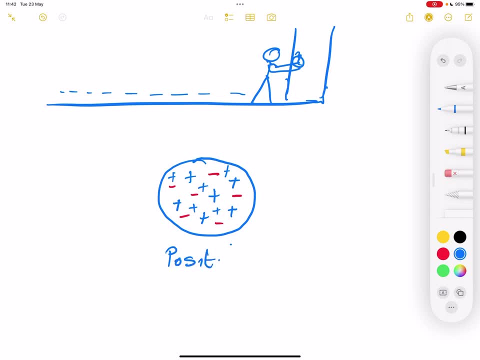 positively charged, okay. I know you guys guessed it correctly, So they become positively charged, okay. So remember again: when I say something is positively charged, all I simply mean is that I've got in this case more protons than I do electrons. It does not mean that there are no. 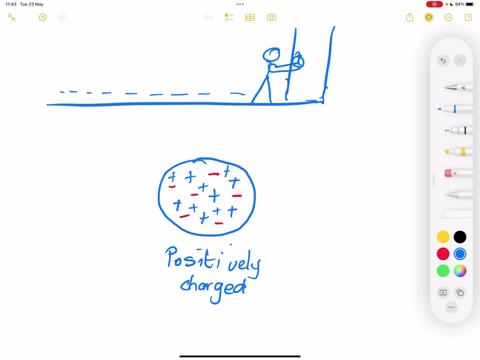 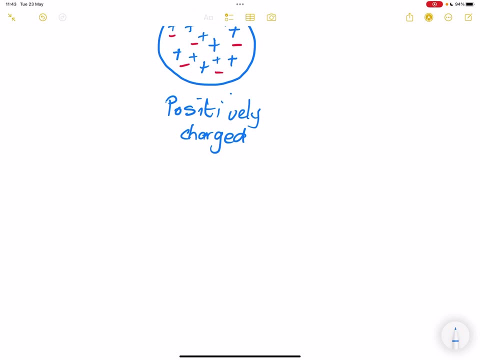 electrons at all. Okay, right, Now we're going to talk about Coulomb's law in just a bit. okay, But here's what we know: Once we've got charged particles, right, they start exerting forces on each other, right. So if I've got a positively charged particle- remember what did we say? positively charged means It means that there's got- we've got- more protons than we do electrons, right? So we say: 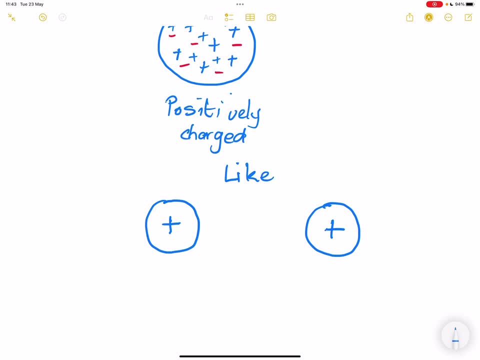 that, like charges, repel each other. So if I've got positive and positive, what happens? They push each other away. The type of force that they exert on each other is a force of repulsion. okay, So this would be a force of repulsion right Now. equally so, even if I were to have negative charges, right? 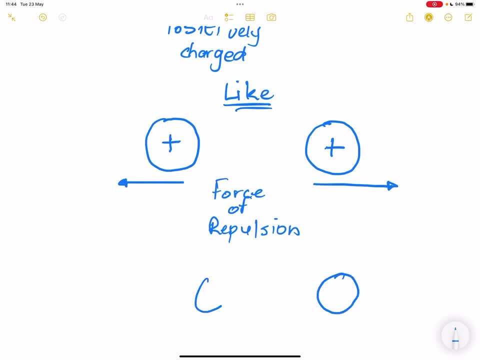 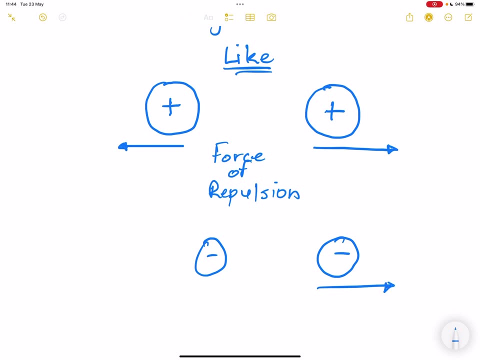 this will exert force of repulsion on each other. So if I do have negative charges, what type of force will they exert on each other? So again, they will exert forces of repulsion on each other. So the moment we've got light charges, we know that they will repel each other. So what happens when we've got? 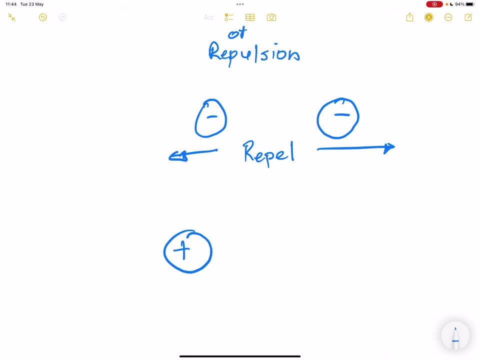 unlike charges, ladies and gents, was this strong feeling her brothers and sisters? So once I've got a positive charge and a negative charge, what begins to happen? Well, Okay, everything succeeds, right. I'm just going to have one more chapter over to symptoms this week. 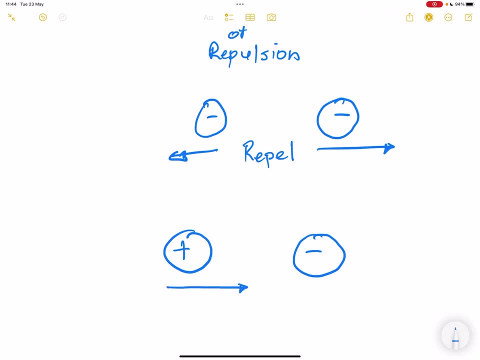 come on. Well, right, we'll start this first talk with you. and What is this? in this case? they start exerting forces on each other, right? And the nature of that force is called a force of attraction. okay, So they will attract each other if they are unlike. 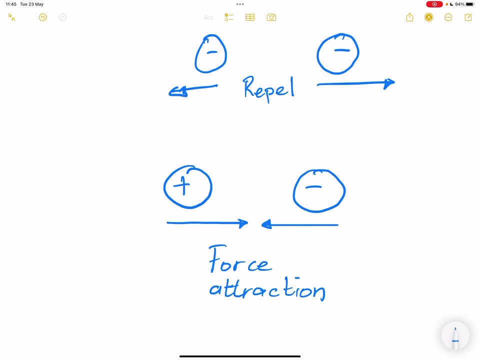 charges. I hope that makes sense, ladies and gents. We'll talk about the nature of that force in accordance to Coulomb's law. okay, Right. So what I just want us to quickly express right now is to talk about- well, in this case, we call it the quantization of charge, right? 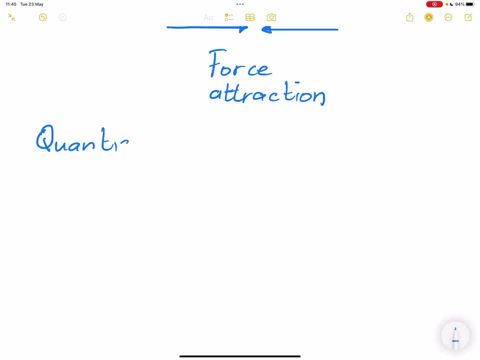 So we talk about quantization of charge. Now that sounds like a big fancy word, right, But when we talk about quantization of charge in this case, we are simply referring to a simple phenomenon, ladies and gents, and I want you to please follow me as I talk about this, right. 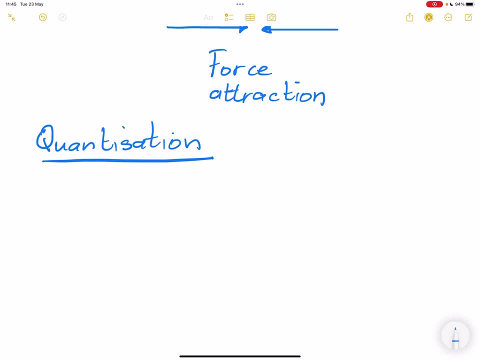 So when we're looking at the word quantization- right So, you can see there there's quanti, right So, which means you are able to get the specific number of something, okay. So what does it mean when we say that a charge or charge is quantized, all right, So, all it simply. 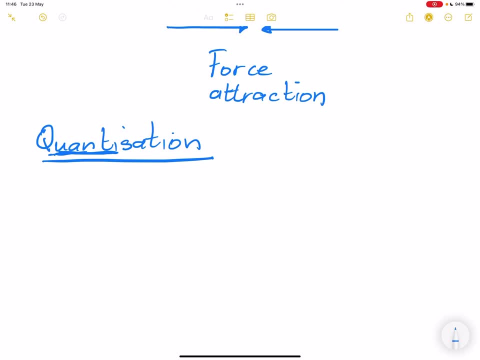 means, ladies and gents, is that, you know, charge consists of, you know, particles, in this case, that are called quantums- all right, We call them quantums, all right- And that you can actually simply, you know, count them, all right. So, in this case, 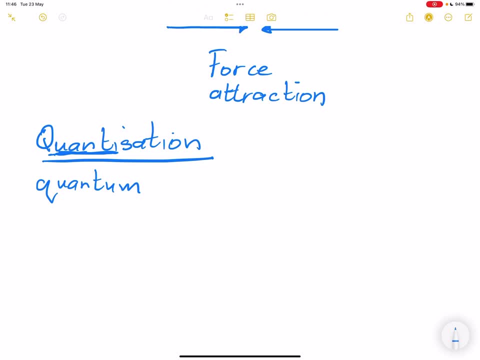 it's made up of, you know, smaller quantums in this case, and they each have a unit. okay, They each have a unit and each unit has got a quantum, all right. So the each electron has got 1.6, or a charge of 1.6 exponent negative 19 coulombs. 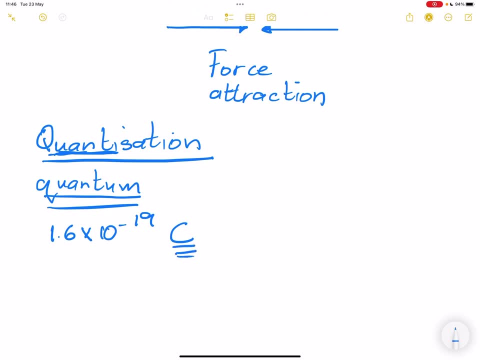 right. So we measure charge in coulombs. Are you with me now, Right? So in this case, that means that every time that I look at a single electron or a single proton, in this case, this would be the amount of charge on them. 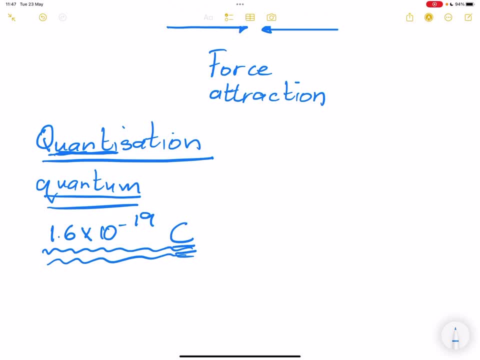 right? So meaning that if I've got multiple electrons right that number, I will see multiples of that number that is given there. okay, So as a result, it means that I can tell exactly how many electrons there are. okay, Right, So in this case, it means that when 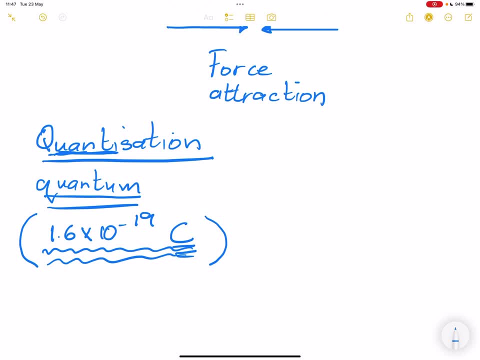 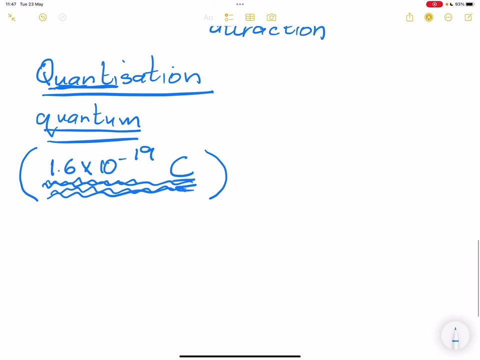 we're talking about a quantum. it's a quantity that cannot be made any smaller. So you cannot get a fraction Of this number right? So it means we can only now get multiples of this number that we are referring to, right? So when we look at electrons, this is the unit charge of a single electron, or a. 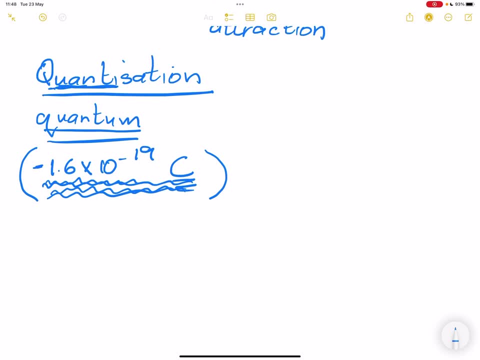 single proton, Of course. with electrons they would be negatively charged. With protons they would be positively charged. All right, So quickly, let's have a look at it. okay, So suppose we've got you know, an object, right? So they give us an object, whatever that object. 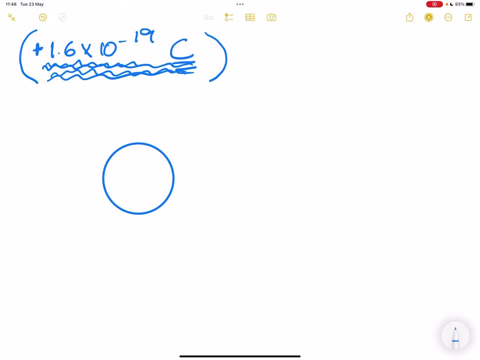 is, it is a sphere, right. And they tell us that, hey look, we've got the charge of this object. let's call it object P. They say to us: well, the object has got a charge of negative 6.4. 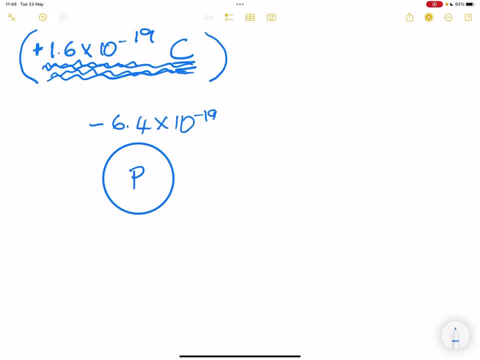 times 10 negative 19 coulombs- right, Sorry, that's coulombs there, right. And they ask us, right, Calculate the number. okay, Calculate the number of electrons that are there, the number of electrons on this object. 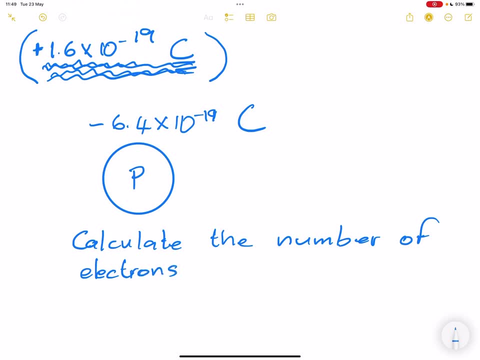 right. So now, what are we going to do? Remember, we know the charge of the particular, you know object And we know the unit charge of an electron. Now note, once it's negatively charged, we said, what does it mean? It means that we've got more electrons than we do protons. So 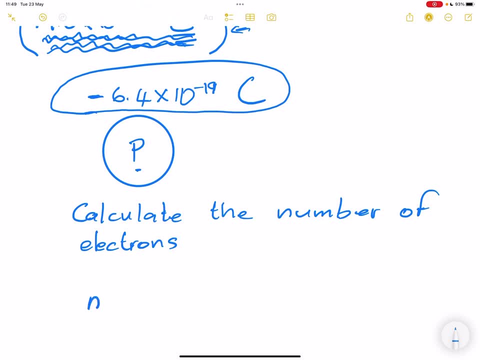 as a result, when I want to know how many electrons there are, I will say: number of electrons in this case will be the charge of the particle divided by the unit charge of an electron. okay, So please keep that in mind. 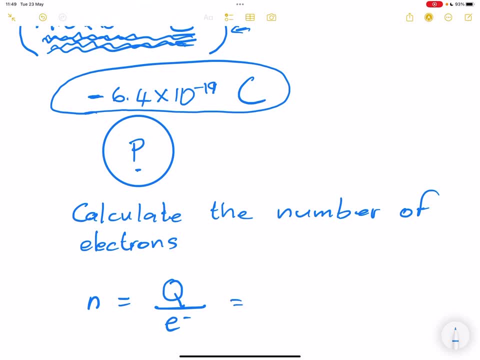 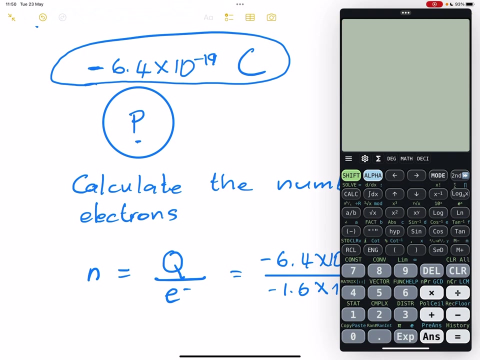 And sometimes they use QE for that. So I will say: well, this is going to be negative 6.4, exponent negative 19, divided by negative 1.6 times 10, to the exponent negative 19,. right, So what are we going to do? Just whip out our calculator, isn't it? 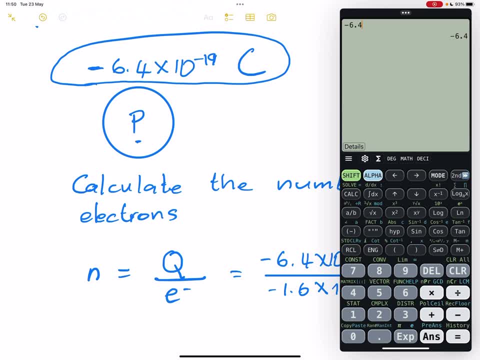 So that's negative 6.4,. right, I'm going to use the exponent button next to the answer button at the bottom right. It's much easier to use than to. you know, use the one. you know times 10 to the power of okay. 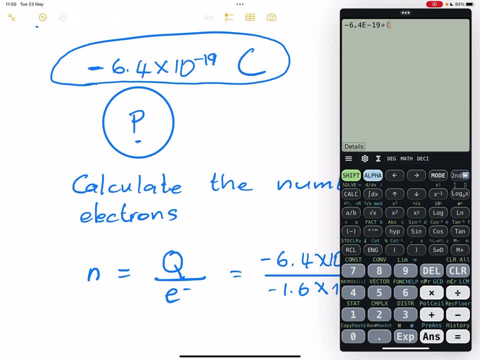 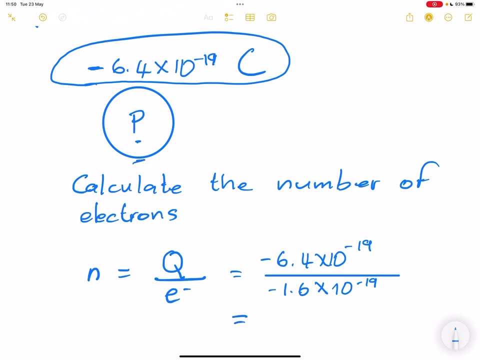 So that's divided by another negative 1.6, exponent negative 19.. All right, do you see that I get a number of 4, right? So it means in sphere P there are actually 4 electrons. Now note, ladies and gents, because we are counting. 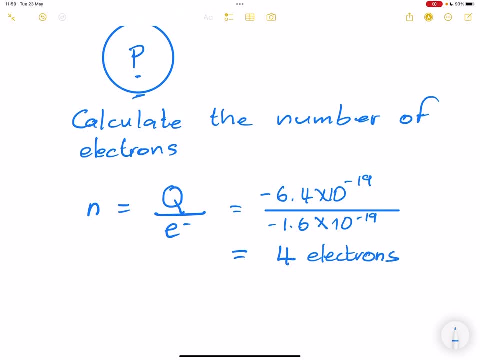 you know actual numbers right? In this case it means we're going to use natural numbers. you know 1,, 2,, 3,, 4, and so on and so forth. So in this case there are 4 electrons in total. 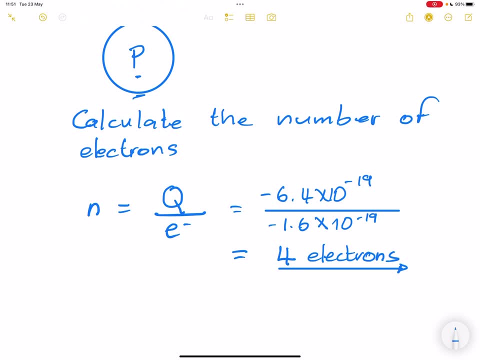 right. So when they say to you, calculate the number of particles, we cannot get a negative number. so that is why, if it's an electron, you're going to use negative, right. so if it's a negatively charged object, you're going to use negative 1.6, but if it's 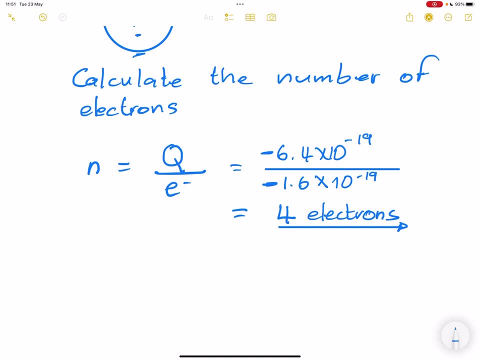 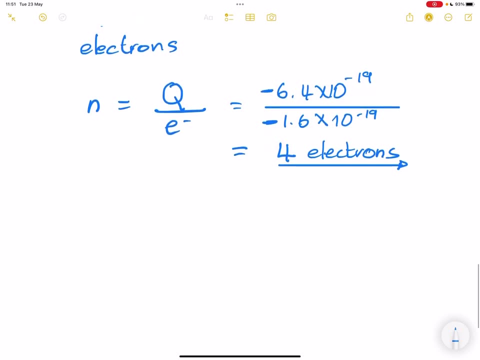 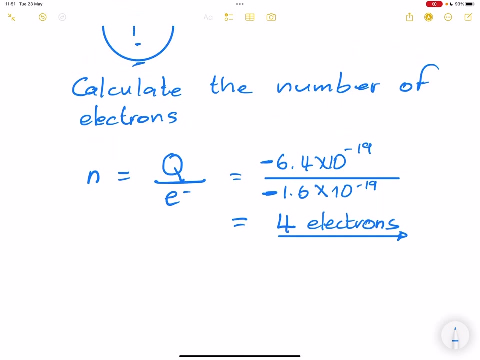 a positively charged object, you're going to use positive 1.6, okay, right. um, i want to kind of delve into something, um, you know, just about the conservation of charge before i conclude, and we're going to look into the next video of it. okay, right? so please remember, we did say 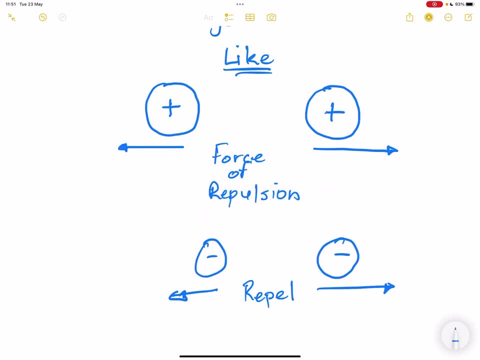 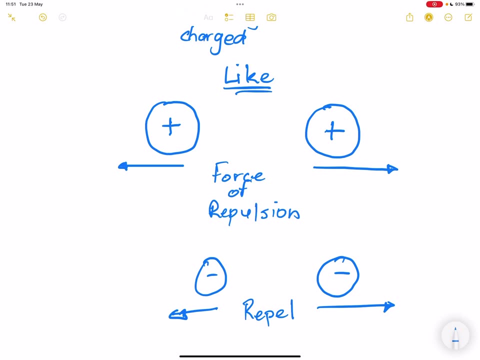 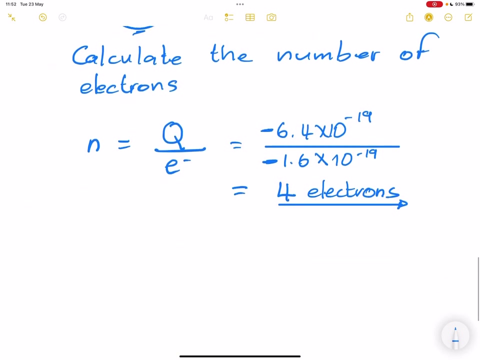 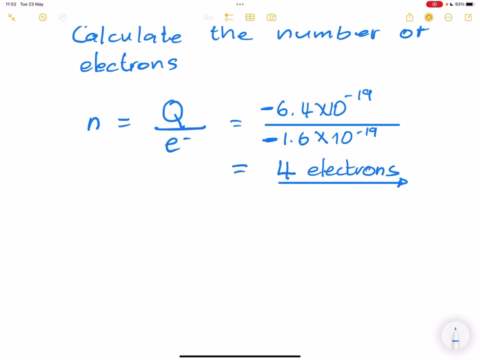 whenever you've got charges that are are the same right light charges, you know we'll experience a force of attraction, of repulsion, rather, and we know that when we've got a force, i mean when we've got unlike charges, then we've got a force of attraction. i just want to look at some symbols that we use right, so i want you to please note. 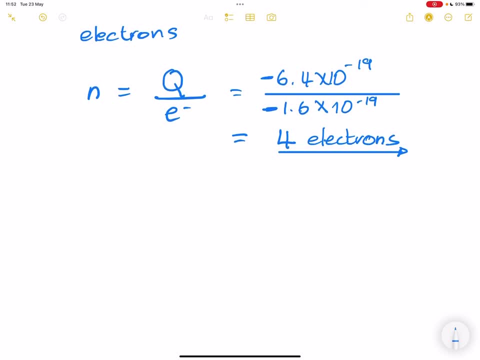 there are some symbols that we use in electrostatics or in physics, um, so i am going to actually just give a little bit of a tabularized format there, okay, so in this table, i'm going to, uh, to give you the name, okay, and i'm going to give the. 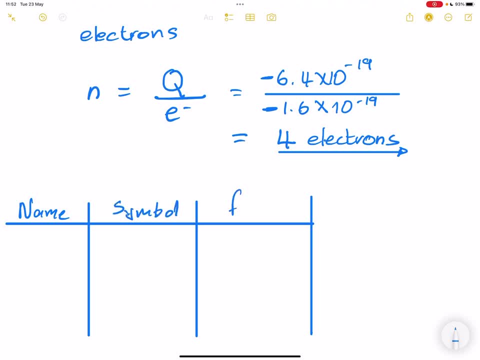 symbol. okay, and i'm going to give the vector so that you know, in this case, what it actually means, right? right, i'm going to start, in this case, with the symbol pico. right, i'm gonna only do the ones that are popular, right? so, uh, we use the greek symbol, pico. okay, so the greek symbol is row there. 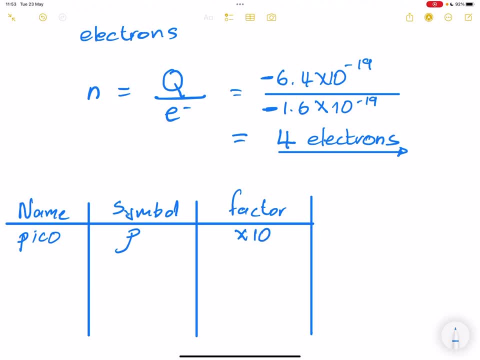 okay, this is times 10 to the negative 12. keep that in mind, right? so when i see the symbol p in this case, i know that they're referring to times 10 negative 12. so we've got nano, right, so we use, you know, that greek symbol there, right? so in this case, that's times 10 negative 9, please. 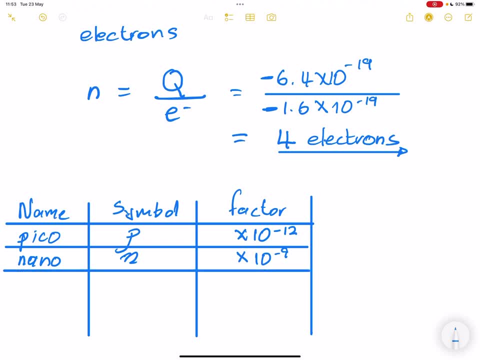 keep that in mind. okay, right, and then we've got um, we've got a micro. okay, and in this case- they like using this quite often- you can say a greek symbol, u, uh, in this case um. or you can actually say, uh, it's the greek symbol. 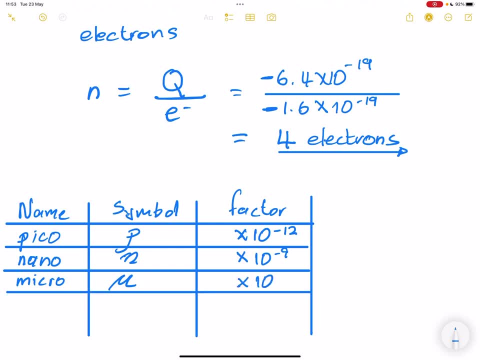 new, right, so that is going to be times 10 um. minus six, okay, and of course we've got other ones, which is um. this is times 10 minus three, okay, uh, all of these, uh, there's be a millimeter or whatever, so in this case we use small n for milli, right, this is times 10 minus three, okay, but you also. 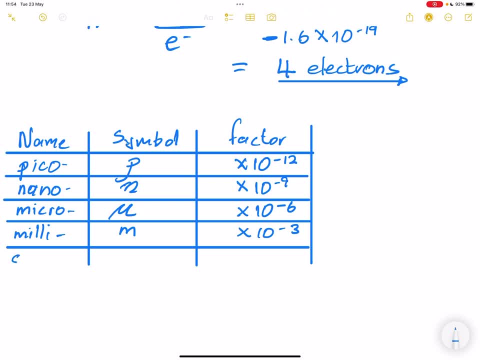 have centi, right, so you've got centi. you know? say, when you say centimeters, you use the small c. this is times 10 minus two, right? or you can just divide by hundred, uh, in this case right. so um that. those are the symbols that we have. of course you do have. 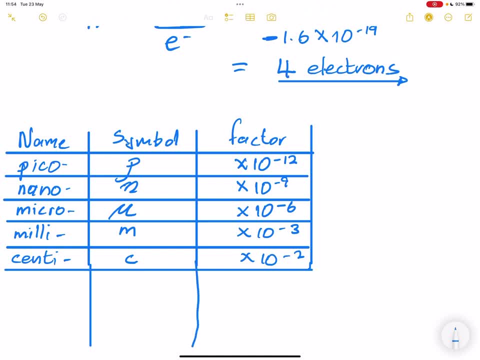 others. okay, uh, we can just uh, continue with that, right? so in this case, we can have a desi. okay, now, when you say desi, that small d, note that this is times 10 minus one. okay, there's a difference between desi and deca, right? so in this case, when you say desi, that's times 10 minus one. 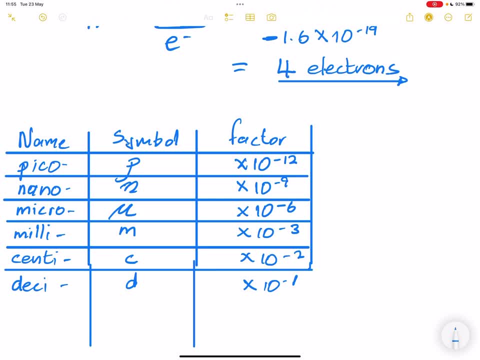 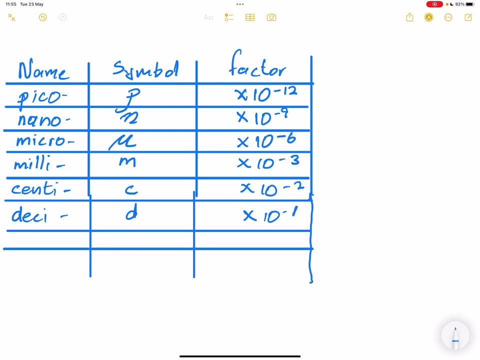 that's why, when you say cubic decimeter, it will be times 10 minus three, because you are actually multiplying it by itself, three times, right? so, ladies and gents, uh, just going to talk about uh, just uh, two more. so, in this case, uh, when we use kilo, right, remember? 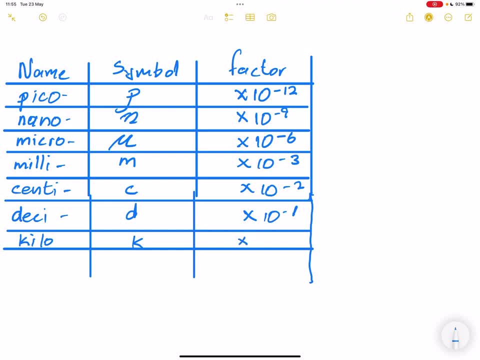 that's that small k and we're going to use kilo right. so in this case, uh, when we use kilo right, we're going to say the right- remember, this is times 10- to the power three. so in this case, it's now positive right and it's positive three. and if you're going to say mega, okay, so we use the big. 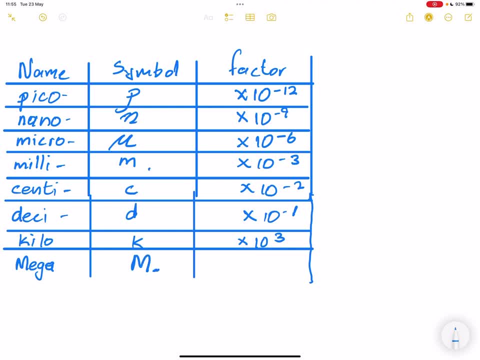 m. note the difference between this one and this one. okay, so mega and milli, right, the difference is the small m and the other one is the big m, right? so mega is times 10 uh to the x bar, so that's one and six uh, in this case you can have obviously giga and so on and so forth, but i'm going to 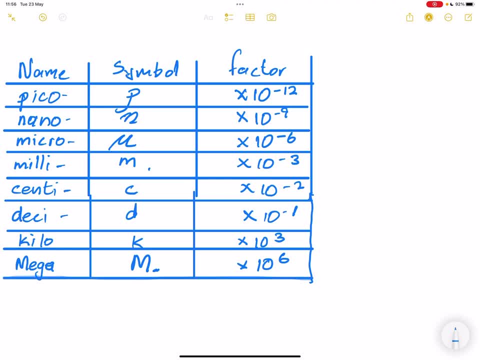 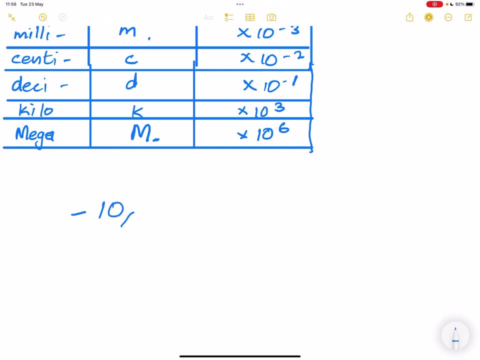 for the sake of our lesson. uh, keep it there, right? so in this case, if i give you a charge and i say this is negative, 10 microcoulombs, right? so then you know this would be negative 10 times 10, negative 6, right? so let me write.